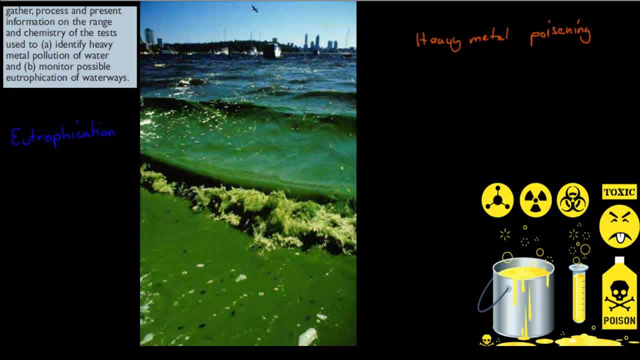 More specifically, we're going to talk about something called eutrophication, which is basically extreme algae bloom Algae are not usually bad, but if they are being grown in big quantities they can cause massive problems. We're also going to be talking about heavy metal poisoning and how we can monitor these heavy metals, and they can obviously come from different industrial wastes. 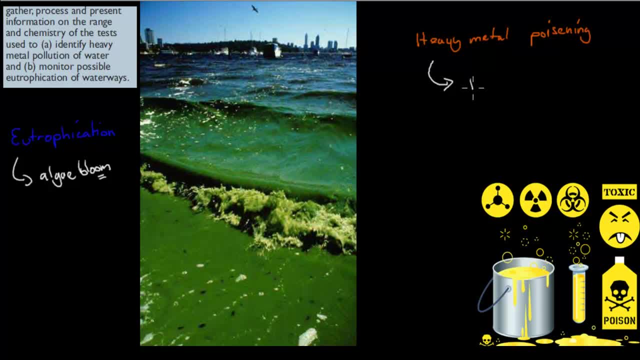 And so these heavy metals, for example, they can cause poisoning in terms of nervous system and also quite a few miscarriages. Different types of heavy metals cause different types of problems, But the ideas that we're going to cover in this video is going to be the following. 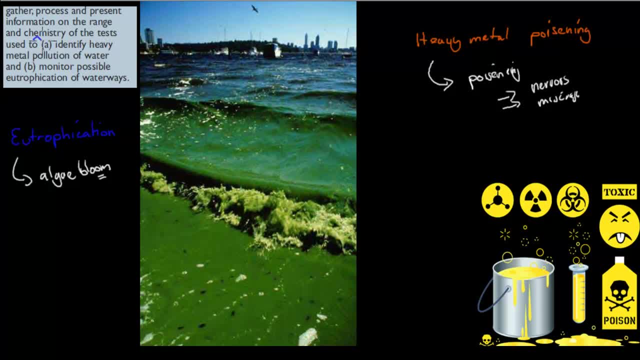 We're going to gather, process and present information on the range and chemistry of the tests used to- A- Identify heavy metal pollution of water and B- Monitor possible eutrophications of waterways. So we're going to talk about heavy metals and eutrophication. 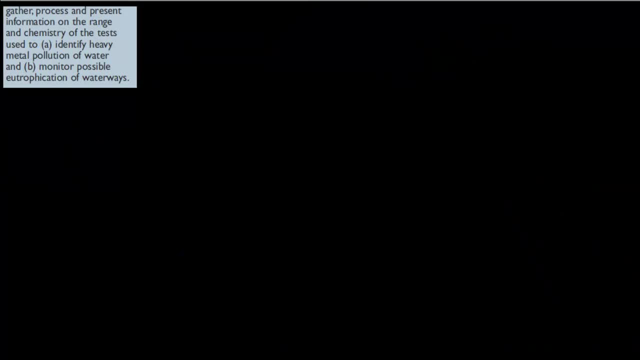 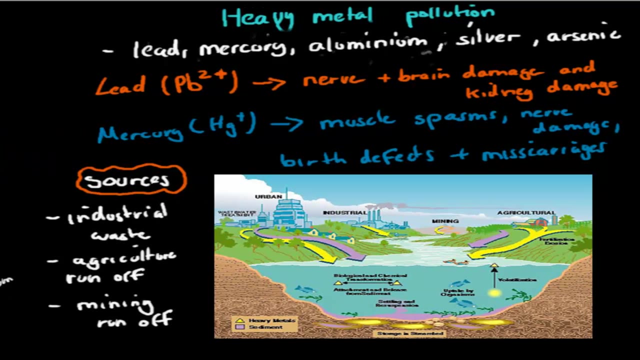 And in terms of the chemistry and range of tests that we can use. So, whilst I'm going to go into a bit of detail in terms of what actually heavy metal pollution is and what eutrophication is, you need to know mostly about the actual tests, the chemistry of the tests and the range of tests that can be used. 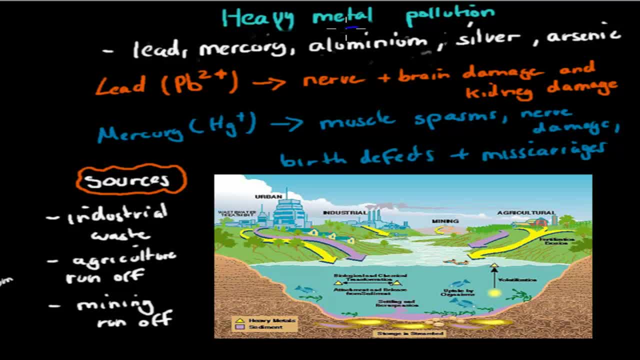 So, for example, heavy metal poison or heavy metal pollution is caused mostly by a couple of different types of heavy metals, such as lead and mercury. These are obviously the two which are probably the most famous or the most well-known: lead and mercury. 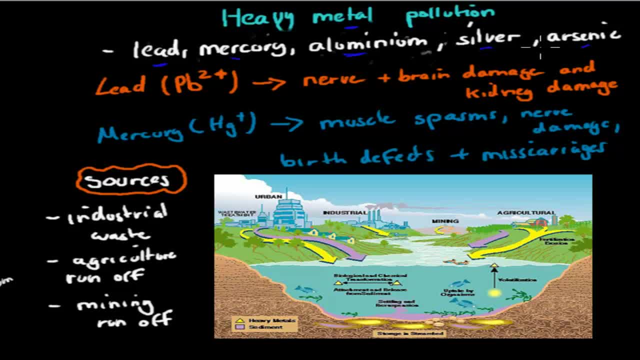 But then you also have a couple of different types of heavy metals, such as lead and mercury. You have aluminium, silver, arsenic, and the list goes on. There's quite a few more, But I'm just going to quickly go over lead and mercury. 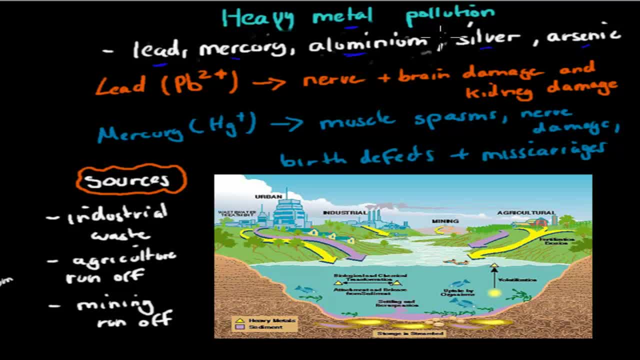 We have actually covered lead in a couple of videos. back We said that, for example, lead poisoning can cause nerve damage and brain damage And on top of that it can also cause kidney damage. So lead poisoning has been a huge problem in the past and it's still a problem in some parts of the world. 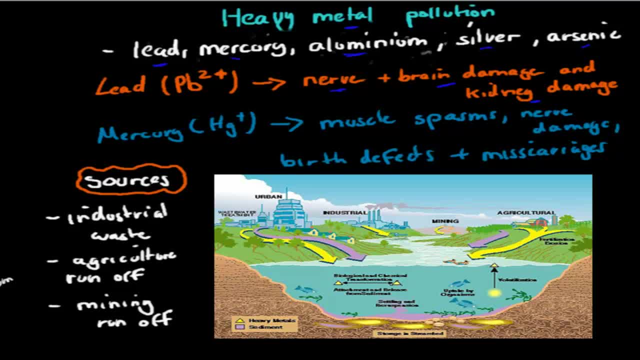 Mercury is also a problem. Mercury, or Hg2+, causes muscle spasms, nerve damage, Birth defects and miscarriages. So again, mercury is also a very big problem. It can also cause lots of problems, And first of all in terms of the sources they can come from: industrial waste. 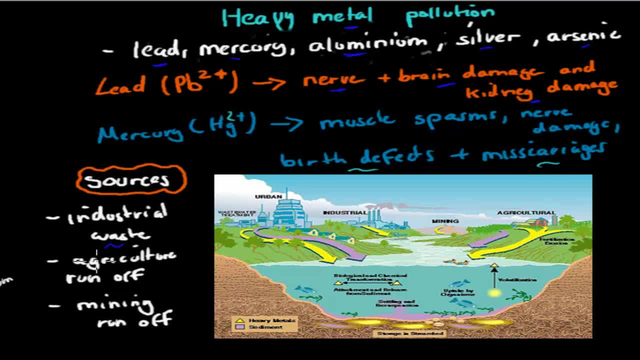 So we talked about how industry might use certain metals in their production and then just dump them into the ocean. There's usually quite strict control over how much, but some of it still ends up in the ocean. Also, agriculture runoff Sometimes. again, agriculture means farming, so sometimes certain heavy metals get used. 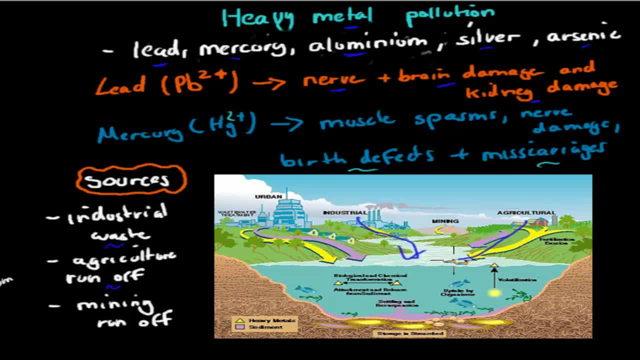 And they just end up in the ocean as runoff. Runoff means running off into the ocean And also mining. so mining runoff, So they might use certain heavy metals for their mining practices or they might be exposing certain mountains or other parts. 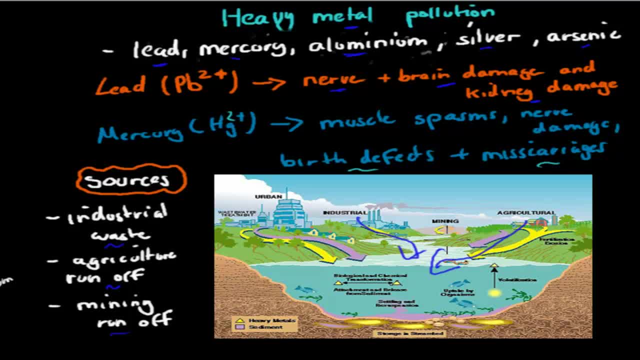 And then you have some of these heavy metals that were in those mountains could end up in the actual river for runoff. So that's what we mean by runoff. So industry, mining and agriculture, all of these runoffs can end up in the actual ocean or river. 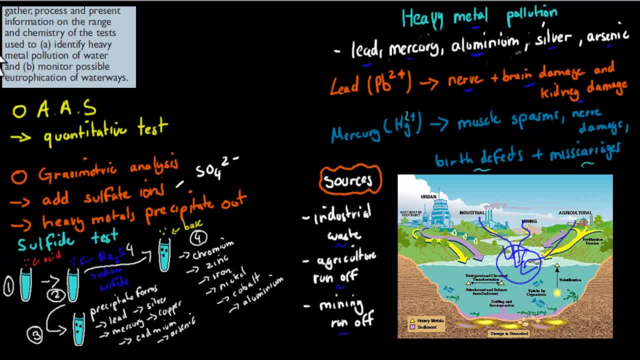 And that can cause heavy metal pollution. But at that point it doesn't say you need to know too much about all of what I just mentioned. But it's good to know And it will be valuable. But what you do have to definitely know is the range and chemistry of the tests involved. 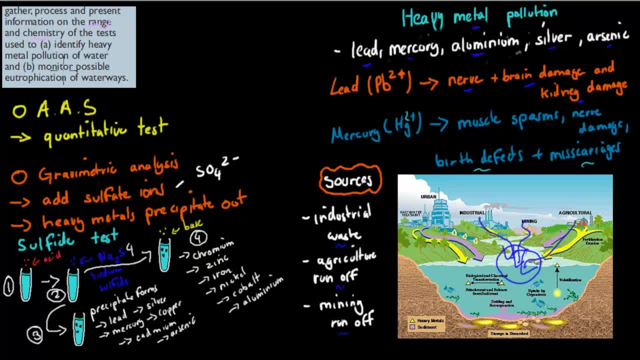 So I'm going to mention three tests and go into a bit of the chemistry for each of those two examples. we have to talk about Eutrophication and heavy metal pollution, But the first test. I won't actually go into detail because you should have covered this by now. 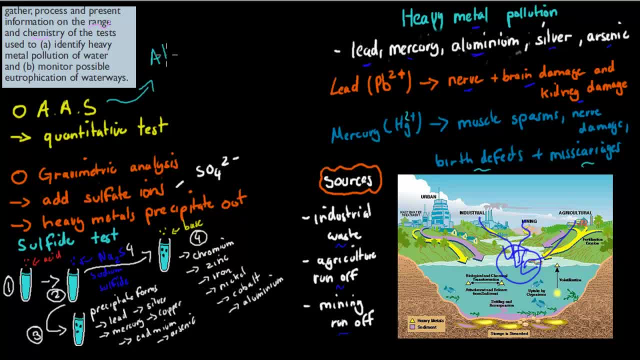 And I've made a video about the atomic absorption Spectroscopy, And so just go over that video, if you haven't forgotten how to do it, Because it can be important. There's a couple of dot points that say you should maybe know a bit about this actual procedure. 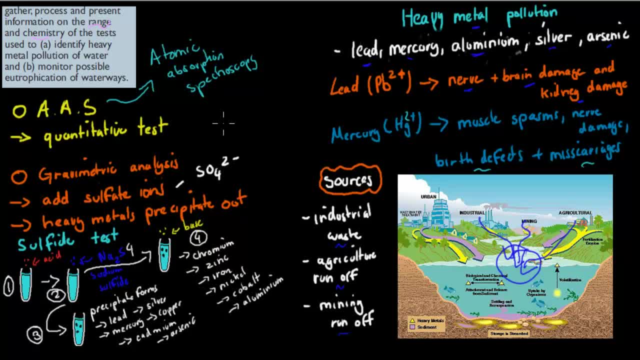 The basic idea would be: you grab your sample, You evaporate your sample, Then there's going to be light passing through And you're going to be aiming to check. if there's, So, the light will be a spectrum. that is, If you're checking for lead, then the spectrum will be lead spectrum. 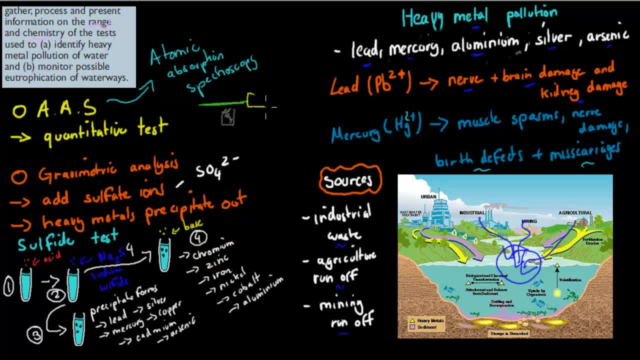 And then you're going to see how much of the light gets absorbed. And the more light gets absorbed, the more actual lead is in that sample. But go over the whole video again if you've forgotten how to do atomic absorption spectroscopy. But this will be one test we can do. 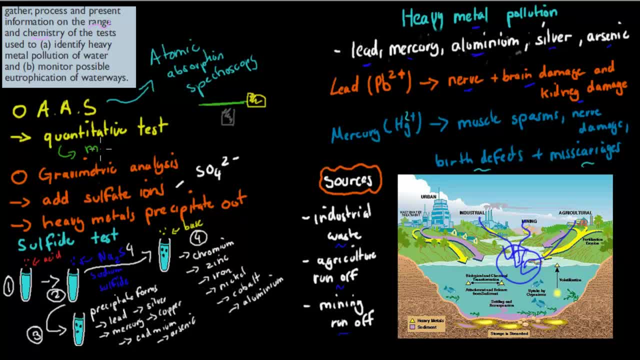 And we can. definitely. This will be probably the most common test that's used to measure for heavy metals, Because, remember, atomic absorption spectroscopy we can use for metals And heavy metals are all metals. Another would be gravimetric analysis, And we combine gravimetric analysis with precipitation. 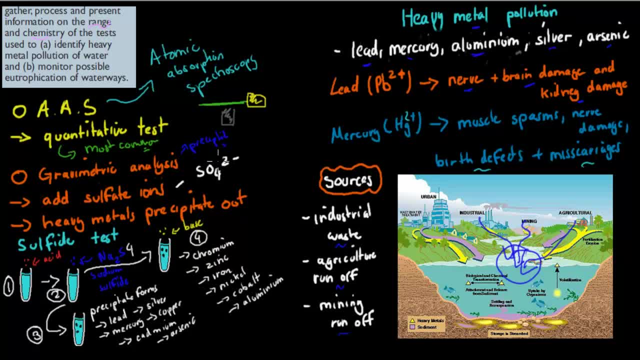 So we precipitate something out And that precipitate. we can then weigh. Gravimetric analysis is weighing. So what we do is we have our sample. So we have a sample And we are going to add sulfate, So sulfate ions, into it. 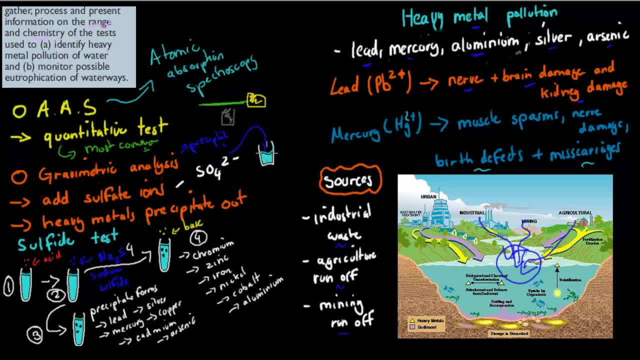 So we add sulfate ions into that solution. So we have our sample. We add sulfate ions into the solution And what's going to happen if there are heavy metals in there? those heavy metals are going to be more likely to precipitate out. 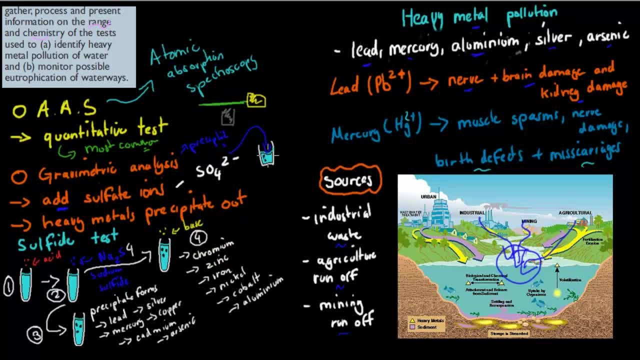 So any precipitate that forms after adding sulfate into that sample will most likely be heavy metals, And then we can weigh those precipitates. afterwards We can evaporate the water and we can weigh whatever that precipitate is And we put it on a scale and then see how much it is. 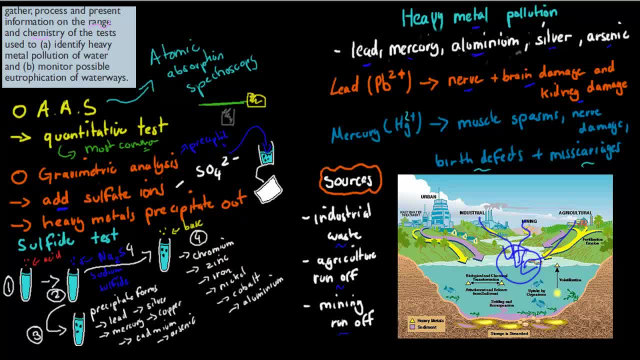 The only problem with this test is we don't know which one, So the question mark would remain about which one are we actually looking at, And also how much of each. It's also not perfectly accurate, because the quantities are often quite small. Small quantities, right. 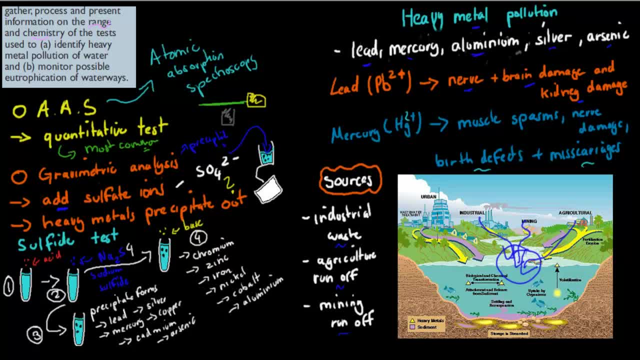 Which is why gravimetric analysis is not really good And we can't distinguish between if it's a lead or mercury or silver, Which is why we often use atomic absorption spectroscopy instead. But another test we can do is a sulfite test. 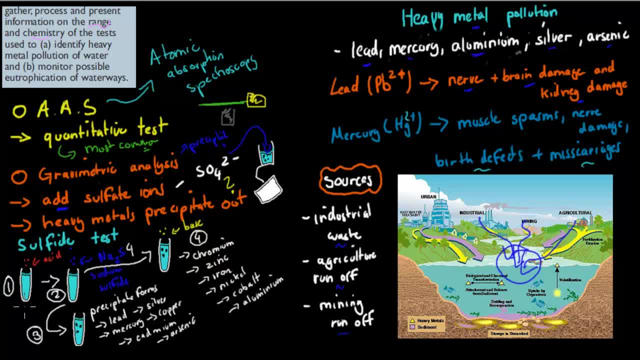 A sulfite test works the following way. So first you have your sample- And this is supposed to be your sample. right here In your sample you're going to add some acids, So you're going to acidify your sample. Second step you're going to do is you're going to add some sodium sulfide. 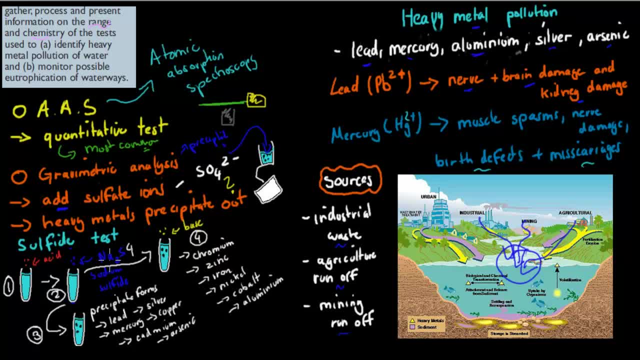 Sodium sulfide is Na2S. Na2S is sodium sulfide. So after putting acid in that solution, you're going to put in sodium sulfide And you're going to observe what happens. Now one of two things will happen. 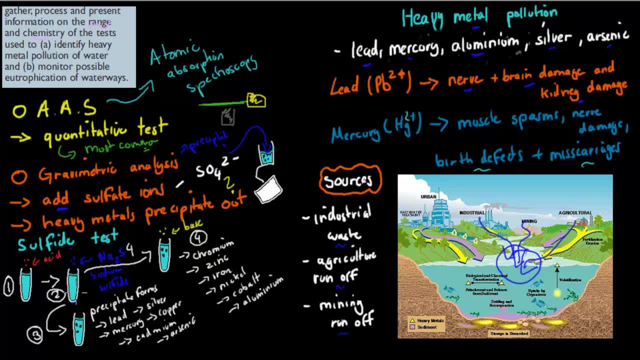 Either nothing will happen or you're going to have a precipitate forming. If a precipitate is formed after adding acid and sodium sulfide into it, that means either lead, silver, mercury, copper, cadmium or arsenic is present. 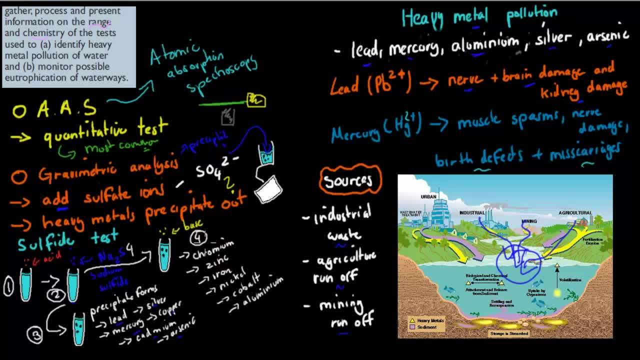 Or, if nothing happens, you're going to have to go to step four. So either something will happen, That means you know these are present. Any of these are present, The precipitate has formed. If nothing happens, you add a base. 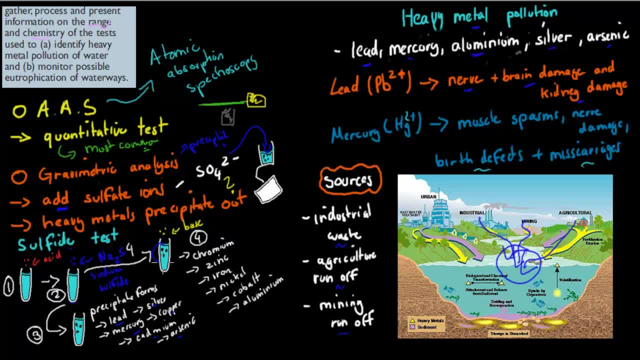 So you make it more basic the solution. And if the precipitate forms after making it more basic, you know that chromium, zinc, iron, nickel, cobalt or aluminum are present. So basically you do your acid in there, You put in your sodium sulfide. 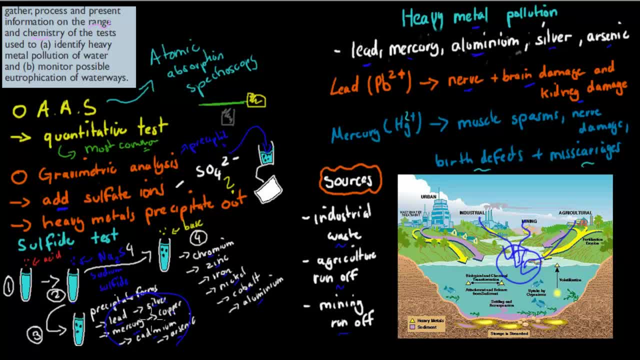 If a precipitate forms, you know these are present. If no precipitate forms, you go to step four, You add base into it, And if a precipitate forms in step four, that means you know any of these are present. So if you want to remember this test, what you should probably do is 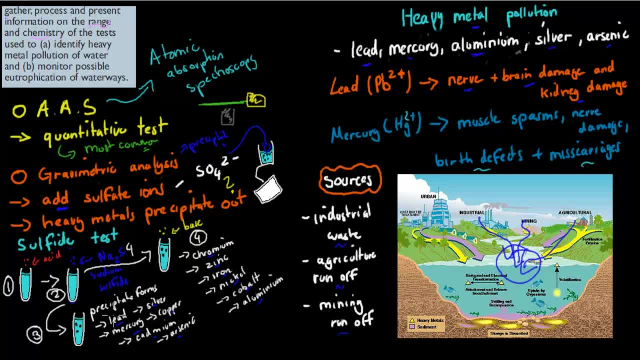 if you can't remember each and every one of those possibilities, just make sure you maybe remember one or two of each step and know just the step-by-step part of it. But these will be three main steps, three of the main tests that you can do. 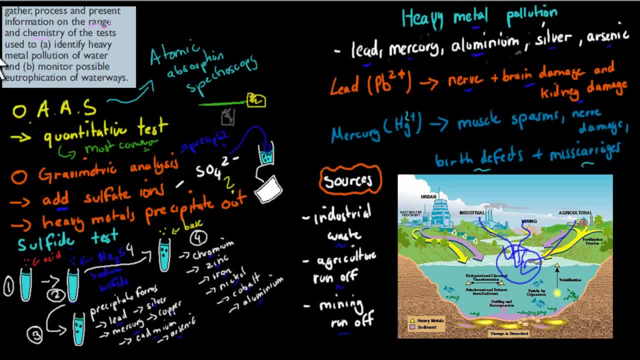 To test for heavy metals And remember the dot point says you need to talk about the range and chemistry of the tests used to identify heavy metal pollution. So I would remember those three names And at least one of them. you should be able to explain the actual chemistry behind it as well. 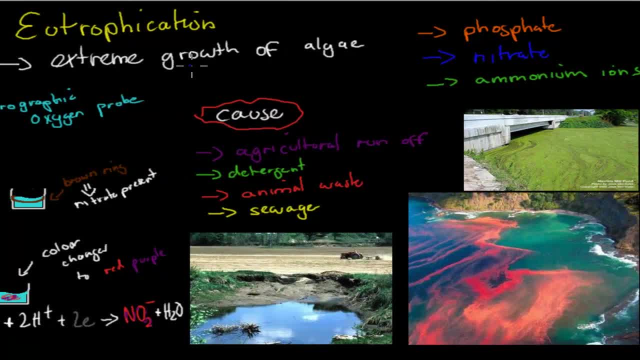 Next one was eutrophication, And eutrophication was the extreme growth of algae. Algae itself is usually not bad, But if it grows to extreme rates that's a big problem, because that means it can kill off. These algae can take away sunlight. 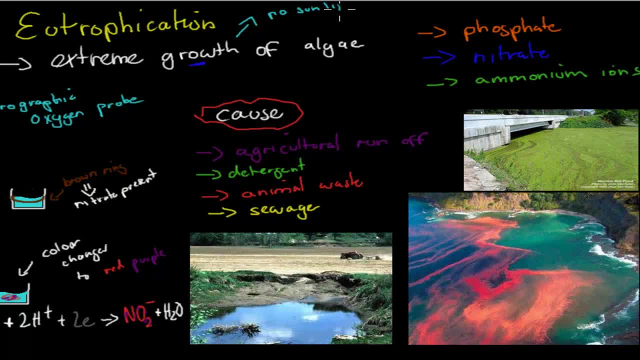 So no sunlight for plants below it, Because what it looks like- it's like this, So you can see- it just grows all over the top of the actual ocean or river. That means sunlight can't penetrate, So it takes away sunlight. It also takes away oxygen. 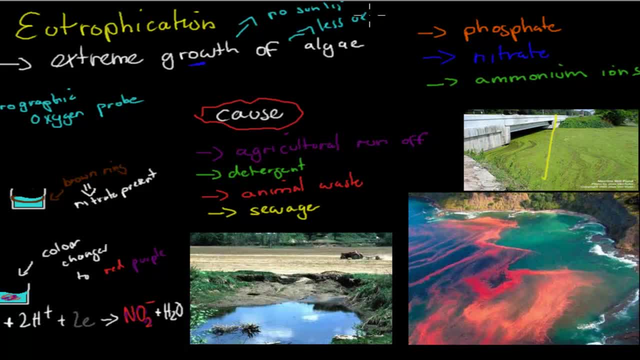 So less oxygen can reach the bottom And again that's another problem as well. So no sunlight, less oxygen would be two problems that would cause eutrophication. So it's bad for marine life, aquatic life, And three things that causes it would be phosphate ions, nitrate ions and ammonium ions. 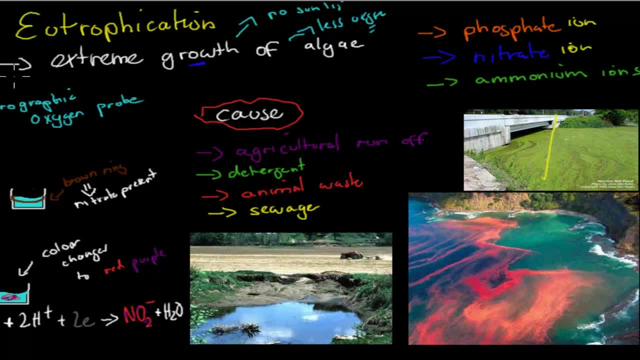 And the reason why is because plants actually need that to grow. Plants and algae need these different ions to grow. So if you give it lots of these different ions, that means they can grow a lot. So basically it's almost like food for the algae. 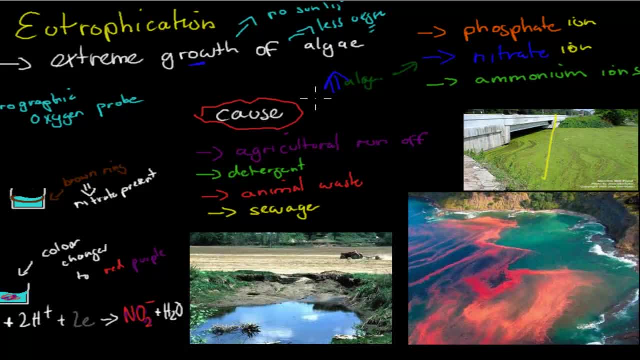 And giving it too much means they will grow out of control, which is why it's called extreme growth. Now, the causes could be agriculture runoff. We mentioned last video. Phosphate nitrate and ammonium ions are released by agriculture runoff. 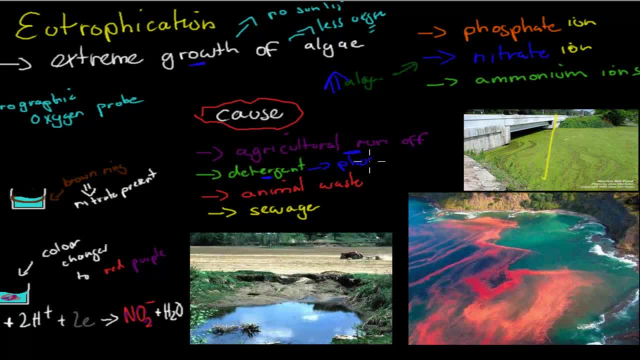 It could be using detergents that have lots of phosphate. Detergents are used to clean stuff, But if you put it down a sink it can end up in rivers- Animal waste. Animal waste has a lot of different ions in there that the actual algae would need to grow. 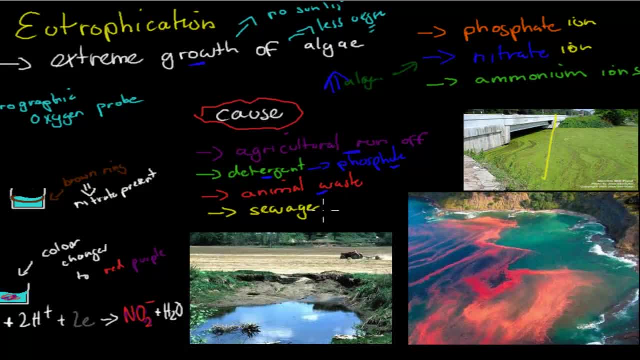 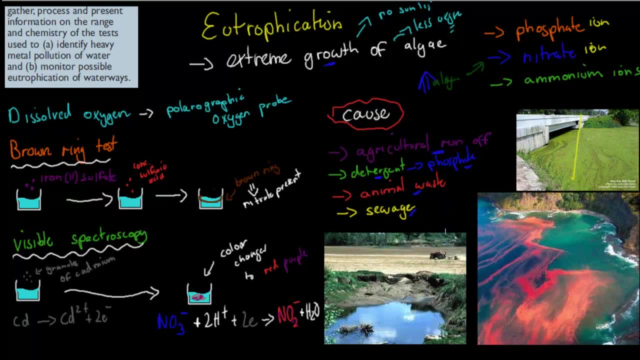 such as phosphate nitrate and ammonia. So if we put animal waste into water and sewage into water, then we have more of these ions in that water And that means we have more algae growing as well, And this would obviously be the idea of agriculture runoff. 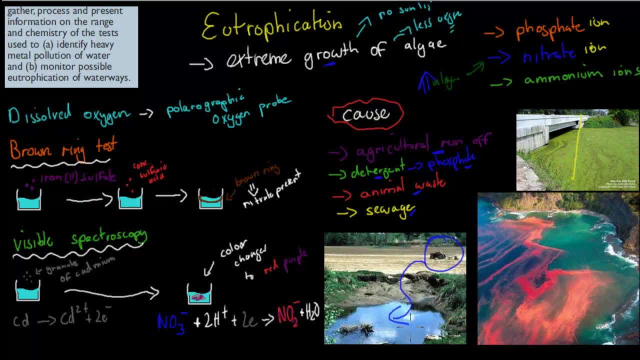 You have a farmer here And then some of the actual phosphate and nitrate and ammonium that they might use as fertilizers could end up in the actual river. So there's three tests again that I mentioned for how to monitor or how to check for eutrophication. 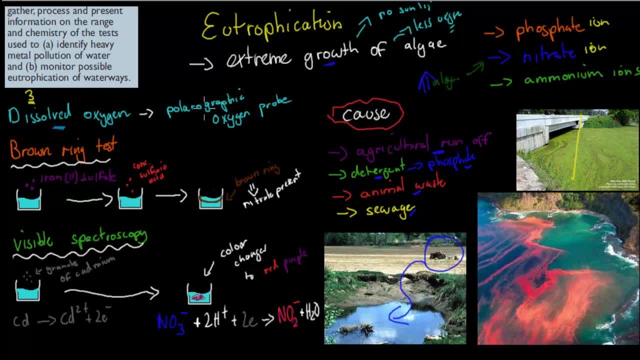 First test would be to check for dissolved oxygen, And remember that was the polarographic oxygen probe that I mentioned in two videos back And that was the idea that we can use oxygen. The more oxygen will complete the circuit and, basically, the more current. 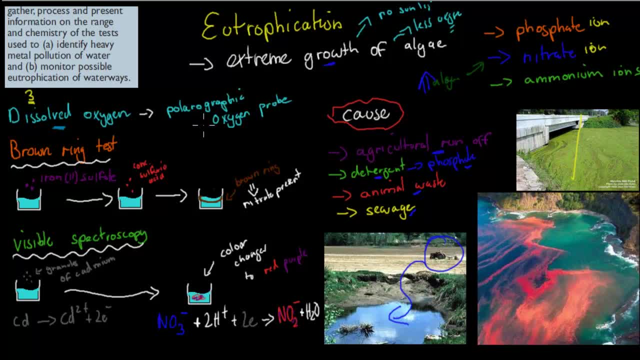 the more oxygen will be in the actual sample, the more current will flow. So we can check by seeing how much current flows determines how much oxygen is there. So that's one way we can measure dissolved oxygen. And remember we want to be able to test that because I said earlier, 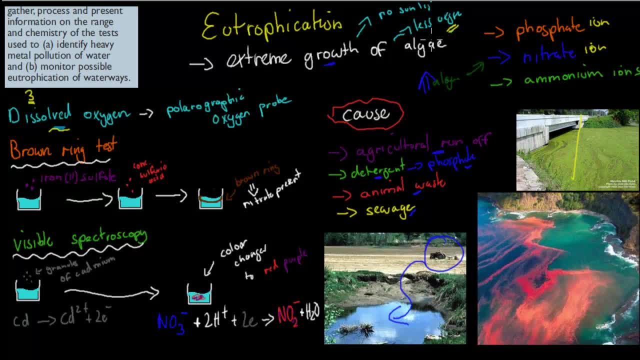 eutrophication. that means there's less oxygen in that water. So by looking at how much dissolved oxygen is in any sample, we can see if there is eutrophication there. So eutrophication would be present if dissolved oxygen is decreased. 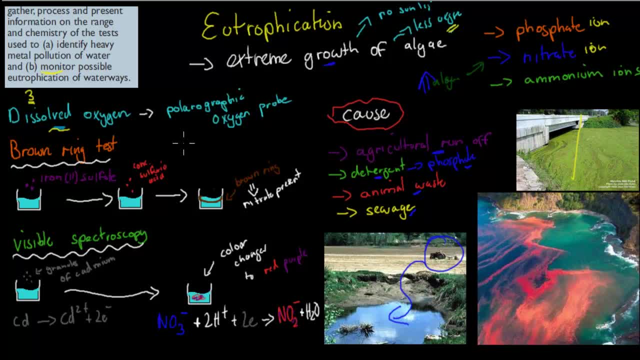 and there's actually one possibility. That's one thing we often do. We test dissolved oxygen and we can use a polarographic oxygen probe for that. But these are two tests I'm going to mention. now I'll go for the chemistry one. They're quite simple. 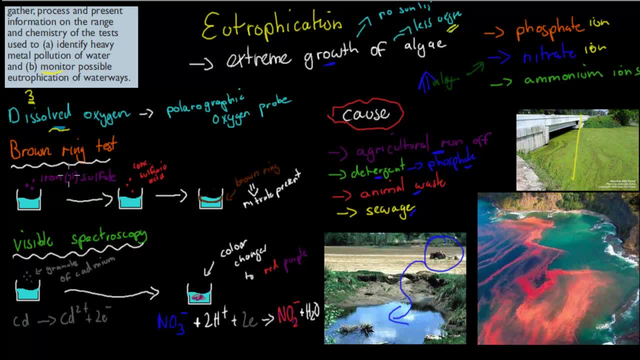 The first one is called Brown Ring Test, and this one is pretty easy to remember because what you're going to have is you're going to have your sample Again. you want to check if there are any phosphate nitrate or ammonium ions in there. 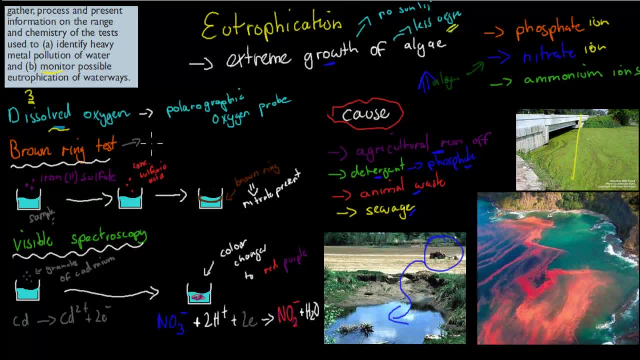 In this case, this actual test will test for nitrate ions. So the Brown Ring Test tests for nitrate ions. So what you're doing is you've got the sample. You don't know what's inside that sample, but what you're going to do is you're going to add some iron sulfate. 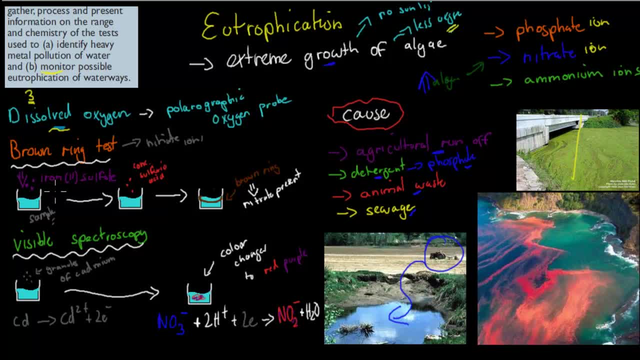 Iron sulfate goes into that sample And next step is, after adding iron sulfate, you're going to add, step by step, bit by bit, you're going to add some concentrated sulfuric acid If you have a brown ring forming around. so, after adding those two things, 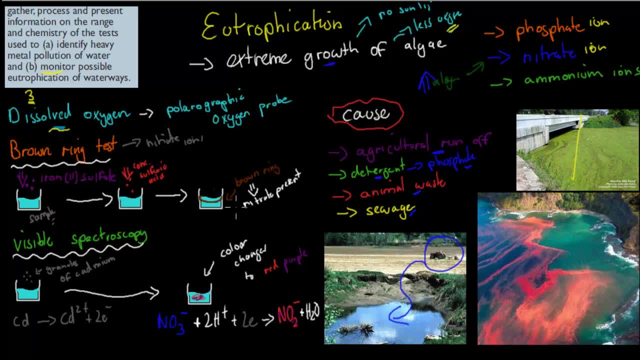 if you have a brown ring forming around the sample, that means nitrates are present. So after adding iron sulfate and concentrated sulfuric acid, if a brown ring forms around the sample, that means you know nitrates are present. That's a Brown Ring Test. 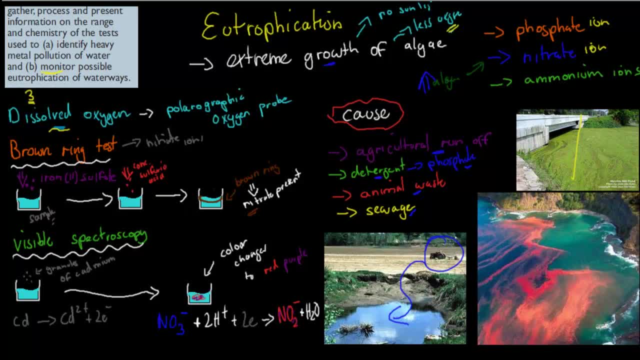 And the other one is the Visible Spectroscopy. And it's called Visible Spectroscopy because what you're doing is you're observing a color change. So what you're having- first you have your sample In the sample. again, you don't know what's inside the sample. 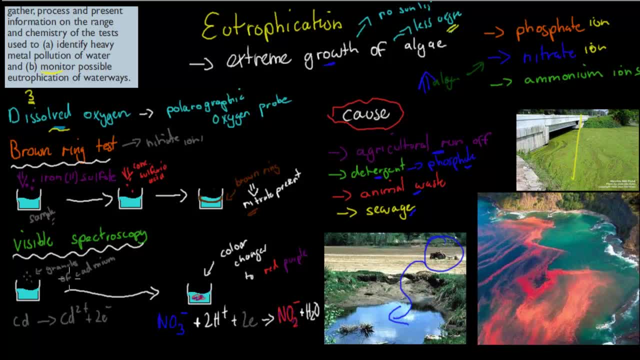 What you're going to do. you're going to add some cadmium first into that sample, so granules of cadmium. Because what happens to those granules of cadmium is they're going to be dissociating. You can see those two electrons come off. 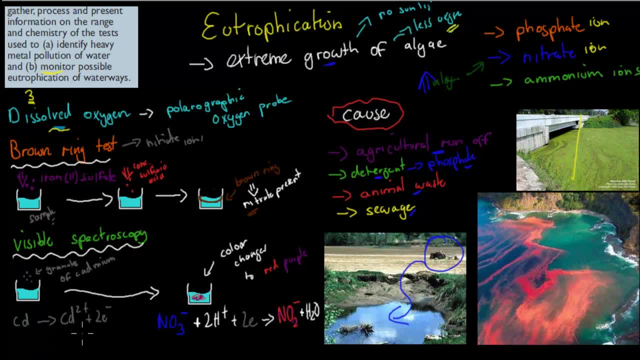 So basically it's being oxidized, Cadmium goes into cadmium 2+ and those two electrons are lost. But if there is nitrate- this is again. this is a test for nitrate, again a nitrate test- If there are nitrate in that solution, what will happen is the nitrate. 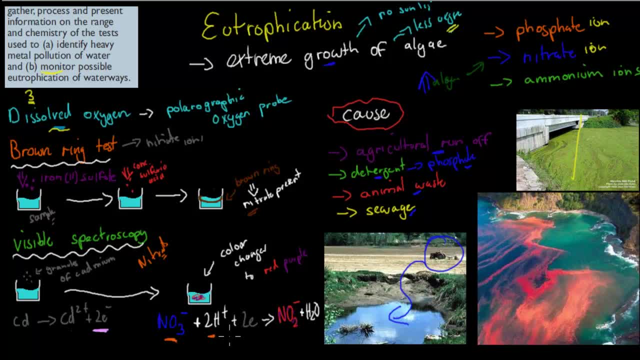 will combine with two hydrogen ions plus those two electrons that came from over here and basically become reduced. So what you can see now is we have formed nitrate. NO2- is nitrate, Nitrate is nitrate and water, But the nitrate will have a different color. 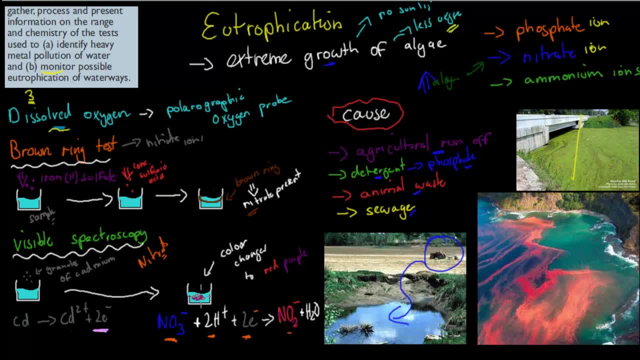 It will have red purplish color. So more or less what has happened here is we have had. if nitrate is present, that means by adding cadmium, the nitrate will take those two electrons and be reduced to form nitrate. 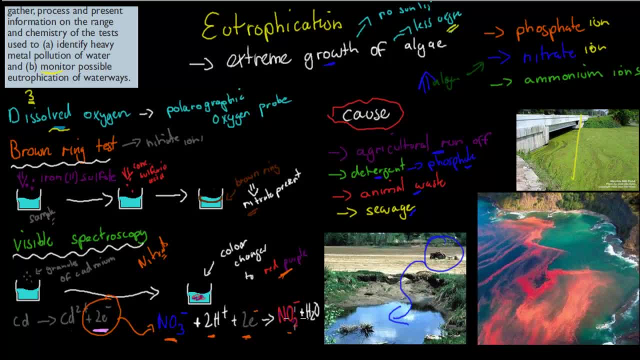 And the nitrate becomes obvious because the color changes to red-purple. So if nitrate is present, that means originally we must have had nitrate, because the actual cadmium must have given two electrons off to nitrate, which is transformed into nitrate. 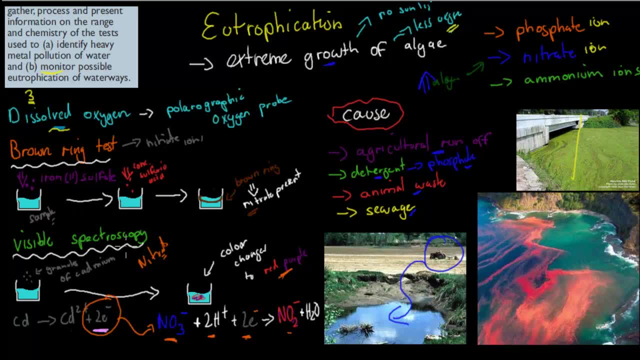 So if nitrate is present, we know nitrate was originally present, so we can use that for a test to check if nitrate is present- And remember nitrate was one of those ions that's needed for eutrophication to occur- 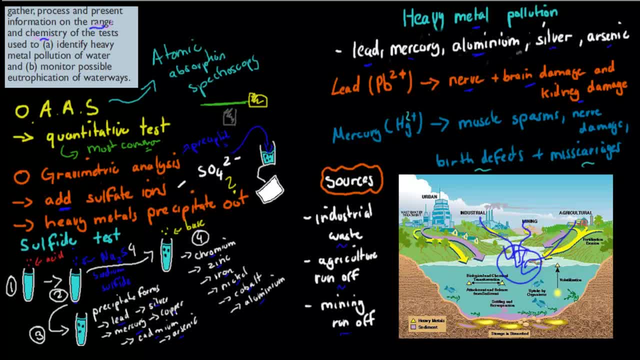 I'll quickly go over some examples. again, We said that to test heavy metals we use either atomic absorption spectroscopy, which was a quantitative test, which means we check the numbers in terms of how much is in there, And this is the most common one used. 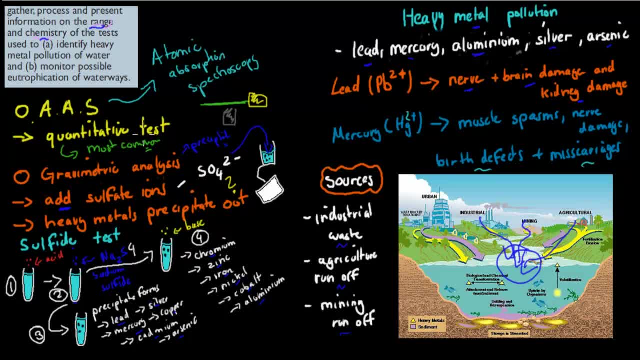 You can also use gravimetric analysis by adding sulfate ions. The sulfate ions will precipitate out the actual, we'll precipitate out the actual heavy metals and then we can just weigh that precipitate Or we can do the sulfide test. 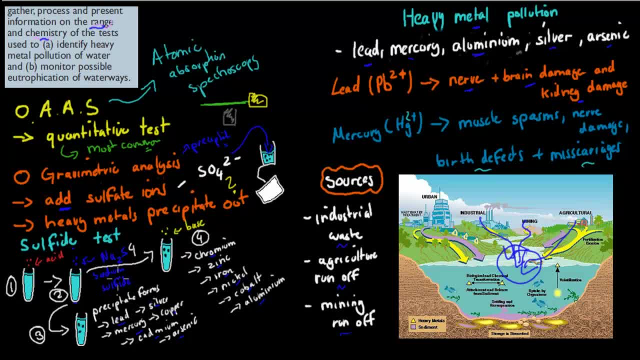 Sulfate test was where we add acid and then, after adding acid, we add sodium sulfide. If we have precipitate forming, we have got either lead, silver, mercury, copper, cadmium or arsenic present. If nothing happens, we go to step four and we add base. 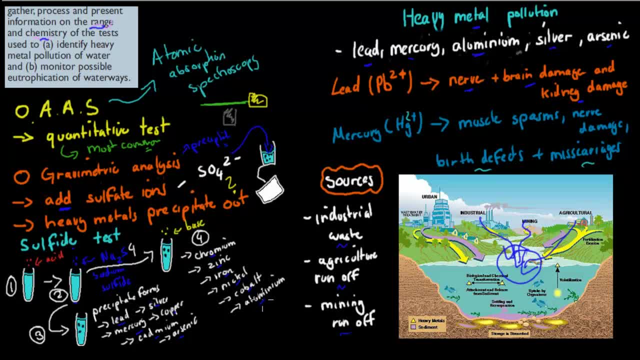 If now a precipitate forms, we know chromium, zinc, iron, nickel, cobalt or aluminum are present. Any of these could be present right. So that's just a test where we can see if we have a range of metals. 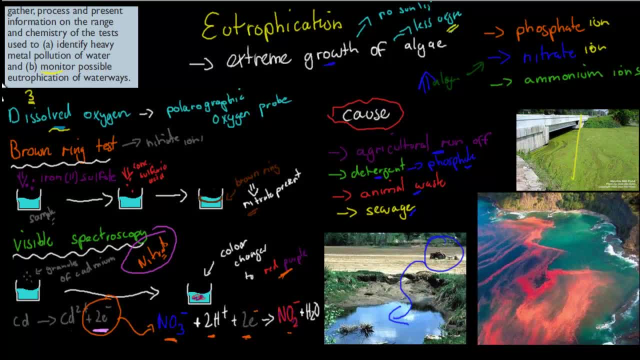 or heavy metals present. And then we have eutrophication. We said we use to check the dissolved oxygen, because we know the less dissolved oxygen the more likely it is that algae booms are present. and we call those eutrophications. 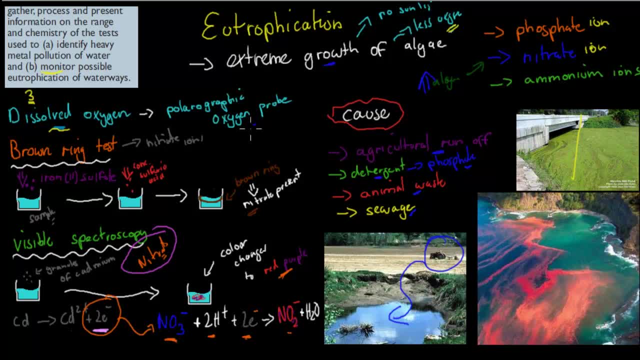 And that was. we used a polarographic oxygen probe to test for that. We can use a brown ring test where we have a sample. we add some iron to sulfate and some concentrated sulfuric acid. If we have a brown ring forming, we know nitrate is present. 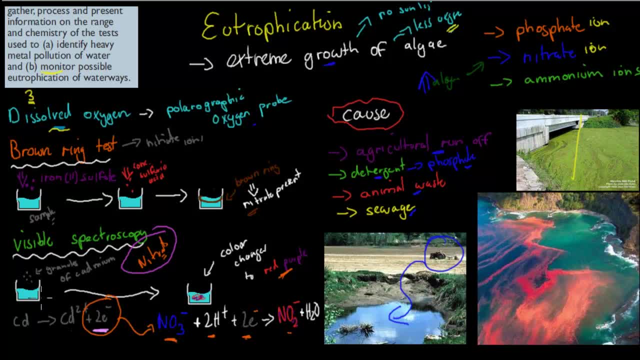 And we can also use visible spectroscopy. where we have our sample. we add some granules of cadmium. That cadmium will lose two electrons because it becomes oxidized in water, Those two electrons. if nitrate is present, nitrate will pick up those two electrons and become nitrite. 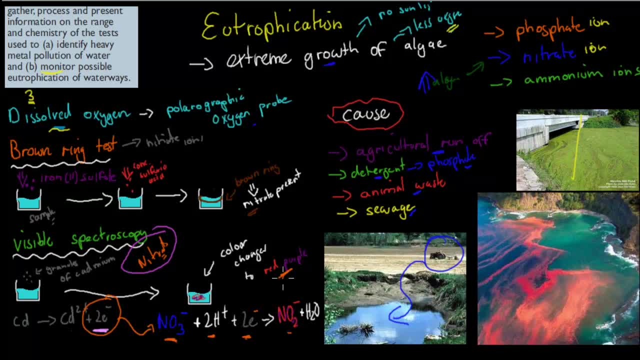 which is NO2- and that nitrite we can see as red-purple because the color changes, And that means we have- originally we would have had- nitrate present, But that's what you need to know for that top one. I hope that was useful.